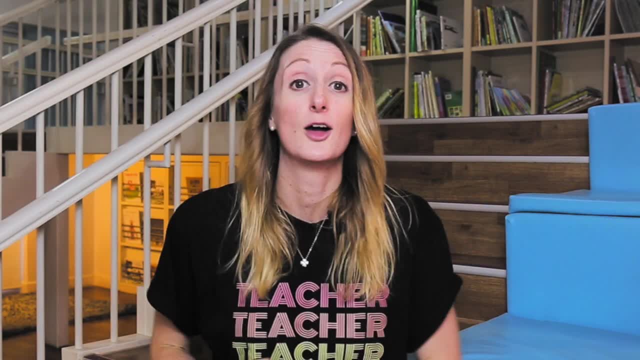 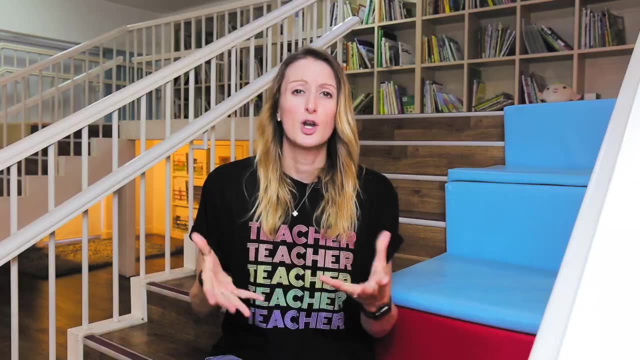 Also real quick. if you are new here, say hi in the comments below and let me know where in the world you're teaching Mathematics. It all starts with the three steps to learning numbers, But not all students find this easy, So we need to find fun ways to practice. So today I want to share a fun 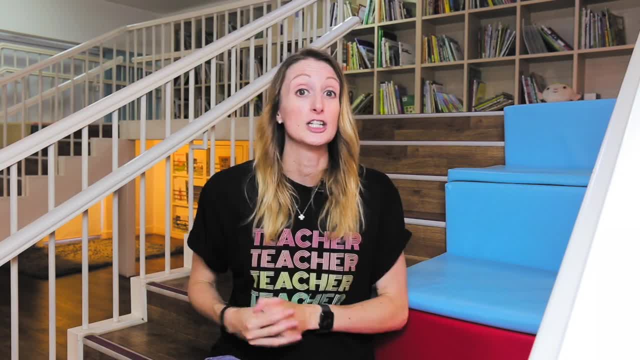 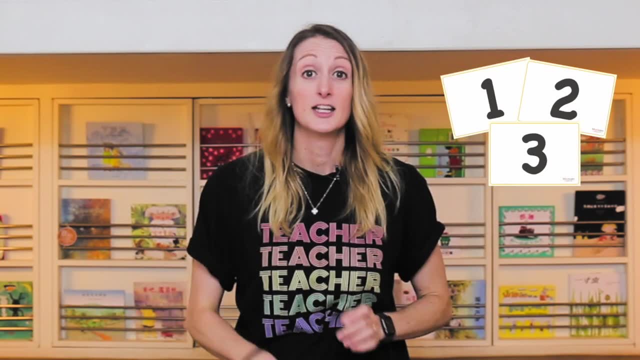 but simple activity to help your students practice number recognition and quantity. So, without further ado, let's get started. For this activity, all you're going to need are some number flashcards, twenty numbered paper cups, some small pom-pom balls and some sort of teddy bear. To get started, you're. 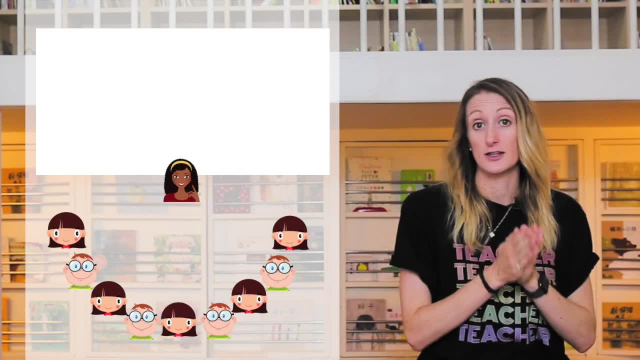 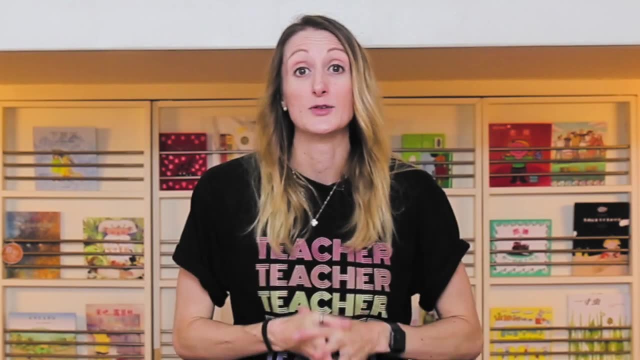 going to position the class in a semi-circle, with you the teacher in the middle. Next, you're going to take those number flashcards and you're going to place them on the board behind you for students to see. First we need to practice root counting using those. 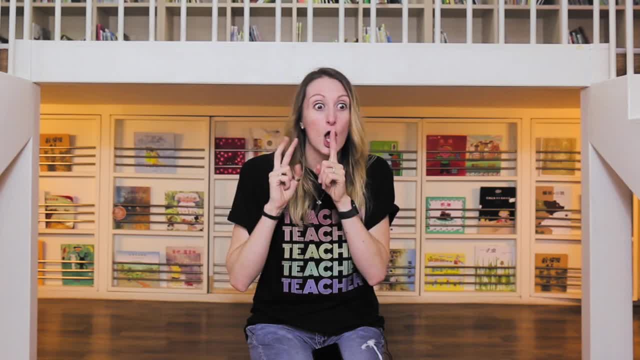 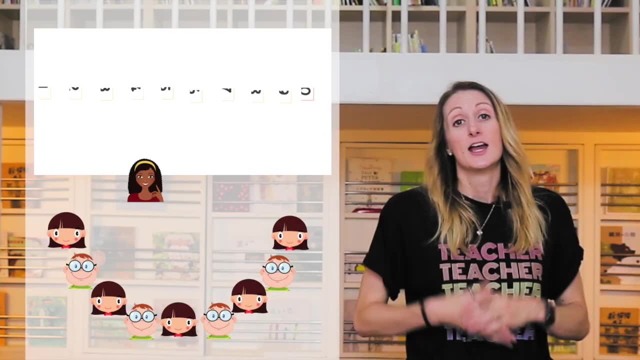 number flashcards. You can make this fun by having students count quietly or loudly, and then, if students are ready, you can have them go around one by one counting in a circle. Next introduce that teddy bear to the class and explain that teddy is sick. But tell them 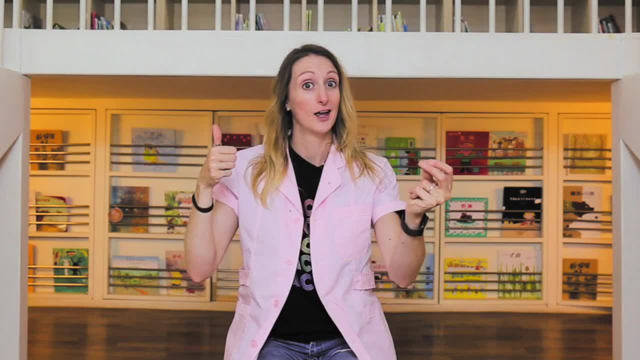 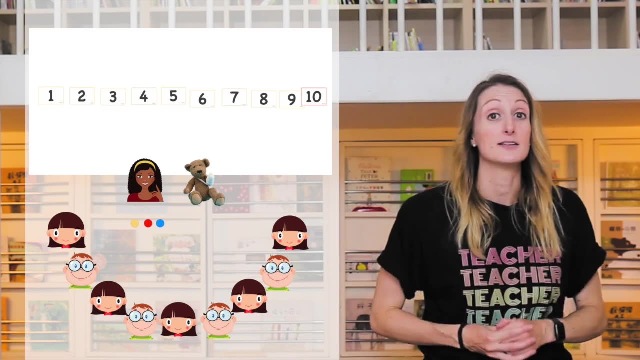 not to worry, because today we're all going to become doctors to help teddy feel much better. Next, introduce those pom-poms to the class and explain that they are in fact medicine balls and that teddy needs some medicine to help him feel much better. Next you're. 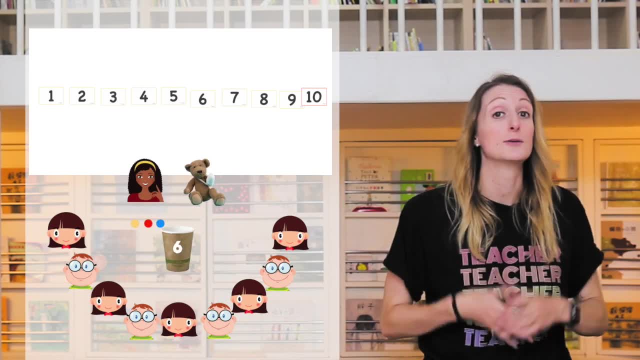 going to choose one of those paper cups, show it to students and ask them what number it is. If students have some trouble recognizing the number, you need to go to the right and that number. then you can use the flashcards on the board behind you as a 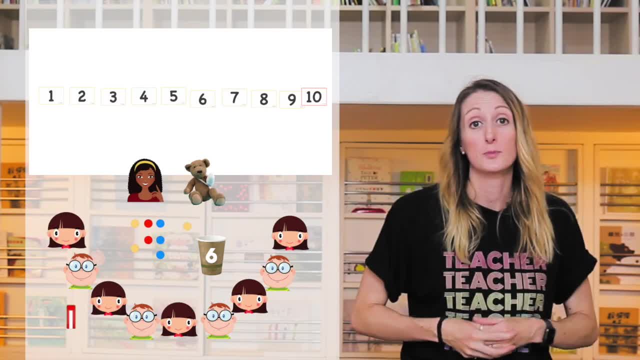 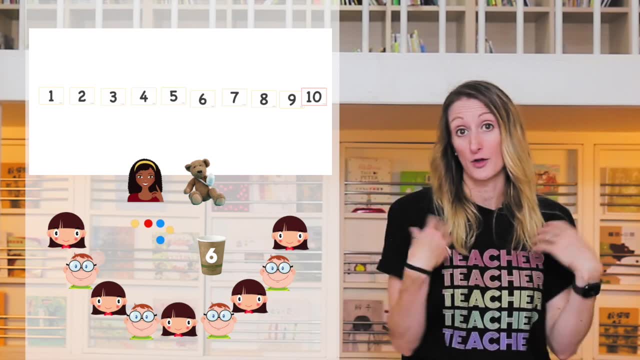 reference. Next, you're gonna count out that number of pom-poms one by one, putting them in the cup as you do. Make sure you are counting one by one and nice and slowly, so that the whole class can follow along. Now that you've shown the 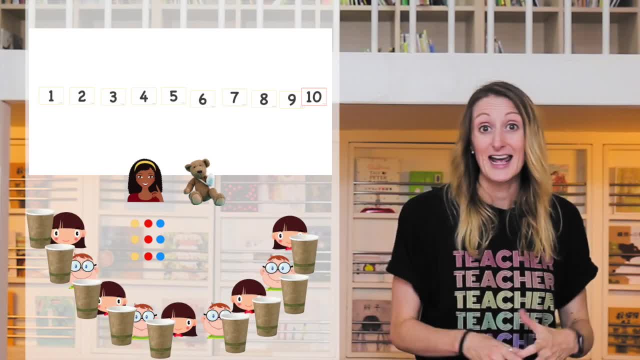 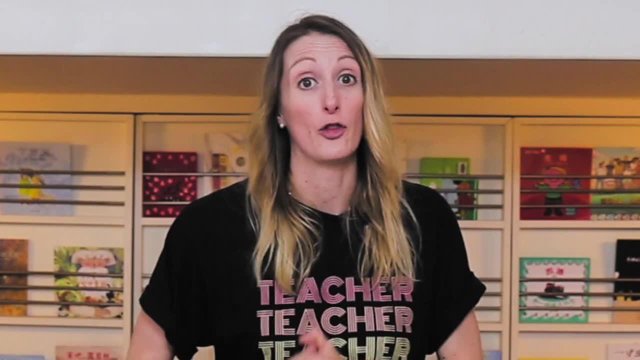 class an example: you're gonna give every student a numbered paper cup and ask them to prepare the correct number of medicine balls for Teddy. Once again, if students get stuck and they aren't able to recognize the number on the cup, then they can use the flashcards on the whiteboard behind you as a reference In. 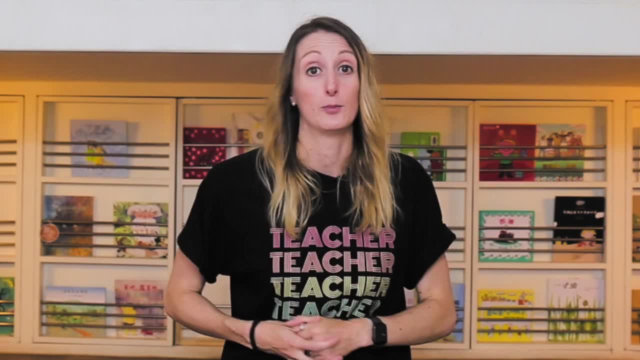 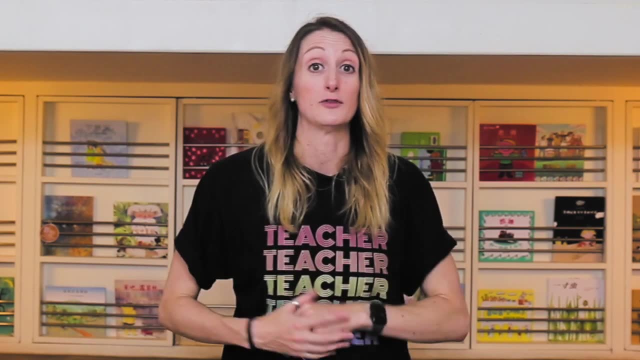 terms of classroom management. you can have students move to tables and have them count the pom-poms there, or you can have them work in groups on the floor. Once they're finished, have them bring their cup with the medicine to the front of the class To finish the class. you can choose one or two of the different cups.